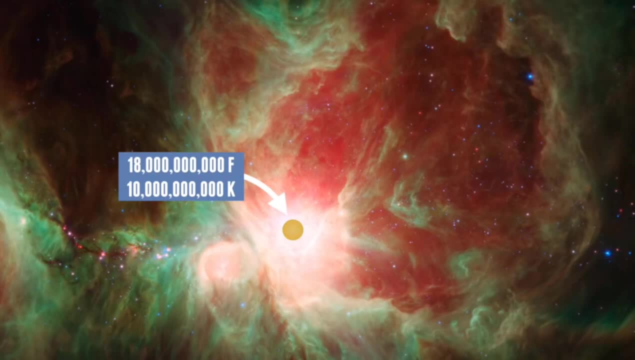 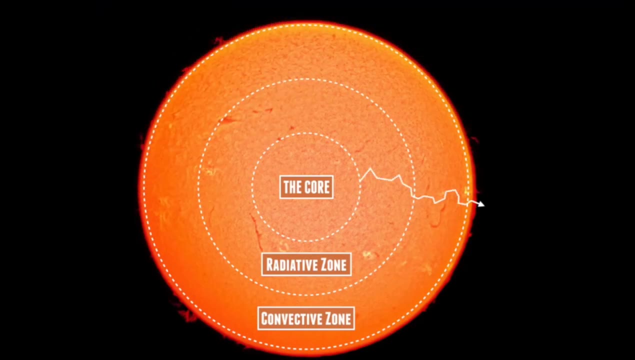 the collapsing ball of gas gets hotter and hotter until temperatures at the middle reach an astonishing 10 billion degrees Celsius. The combined energy released by billions and billions of individual fusion reactions flows outward from the star's core. Some of it eventually emerges from the star's surface as light. 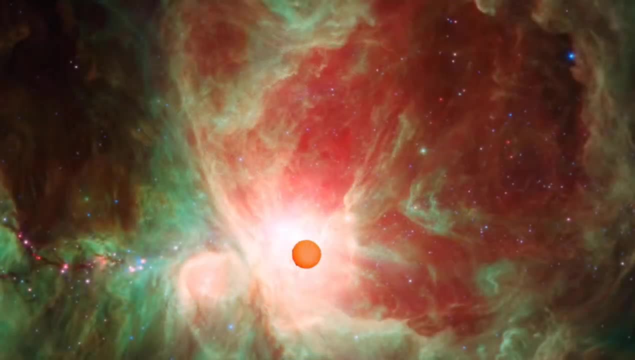 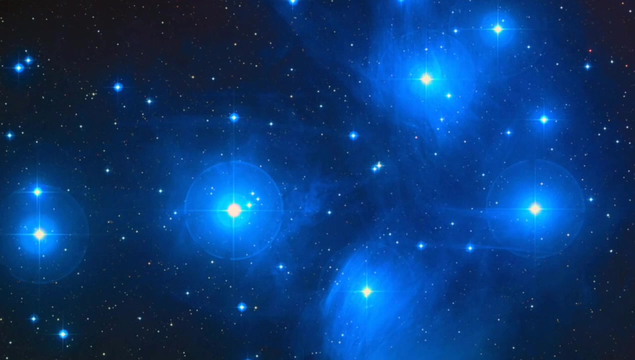 light, along with particles blown off the surface of the newborn star, sweep away from the surrounding cloud of gas and dust and therefore a star is now born. Most stars are born in groups. these are often called star clusters, Clusters like this that stay together. allow us to track the stories of the stars. while less massive clusters will simply dissolve because of the lack of gravity, These stars in less massive clusters will eventually mix into the general population of the Milky Way. Most stars will simply wander the galaxy until they get into a stable orbit, very similar to how a planet orbits a star. 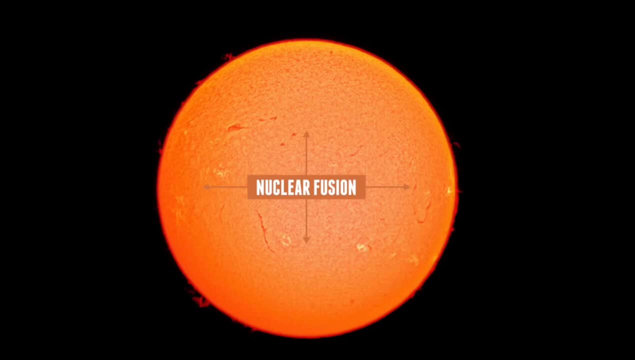 The outward push from nuclear fusion in its core is now nicely balanced with the inward push of gravity, and the star remains in this balanced state for about 90% of its lifetime. This is now at the stage that the sun is now in It's. 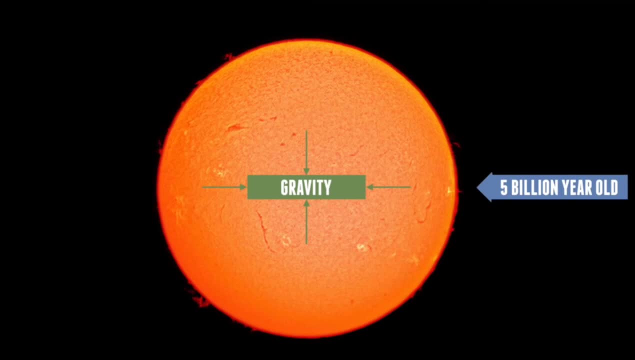 been at this stage for almost 5 billion years, and it will continue to do this for at least another 5 billion years more. Having a stable star is thought to be critical to the development and evolution of life. How long a star lives depends on how much material or mass it has. 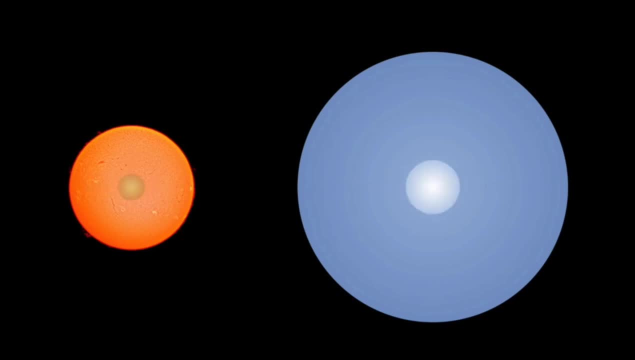 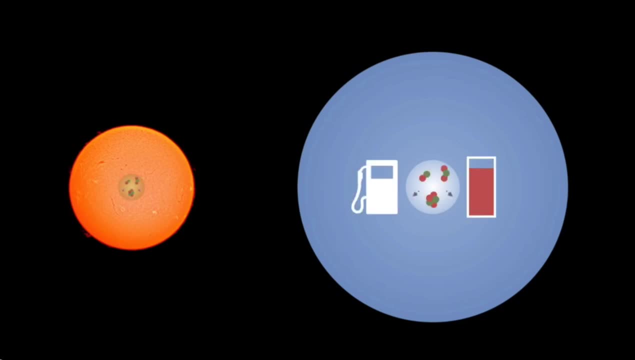 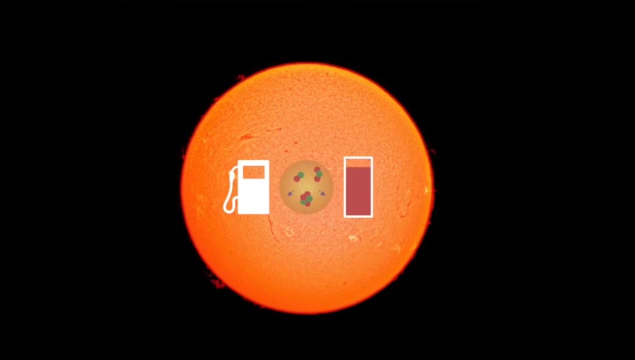 hydrogen atoms extremely fast and exhaust their fuel very quickly. The most massive known stars last only a few million years. The core of the lower mass stars, like our sun, is a lot less hot and burns its fuel a lot more slowly. 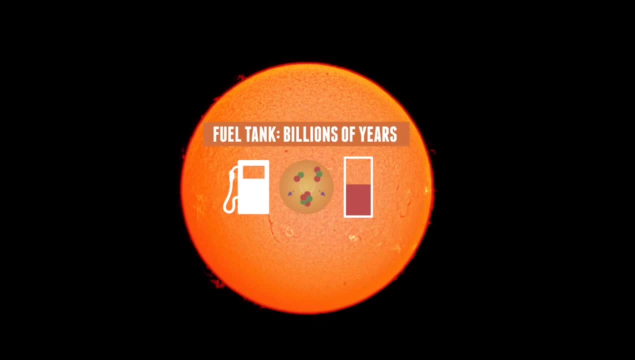 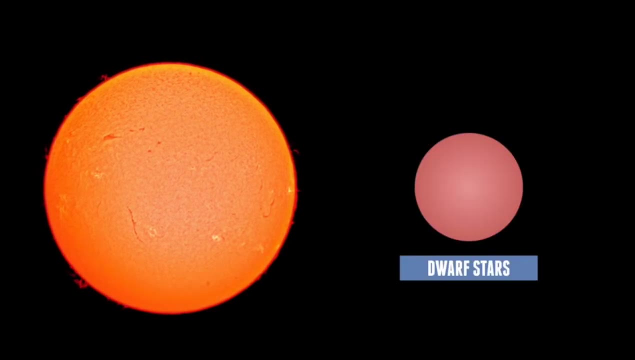 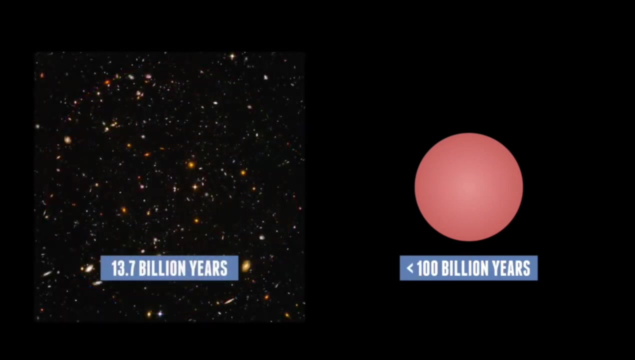 This means that our star can last for billions of years rather than just millions. The lowest mass stars, known as the dwarf stars, burn very, very slowly and they may last more than 100 billion years. This is much longer than even the current age of our universe. 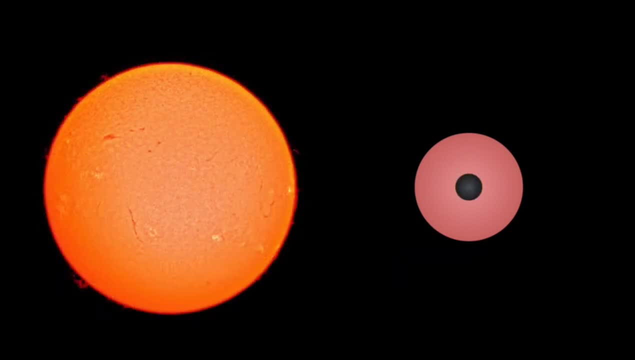 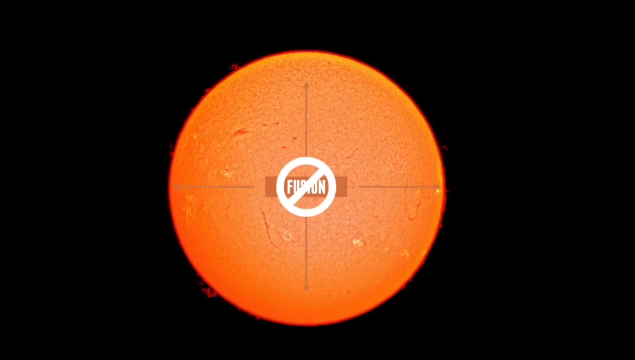 Nevertheless, the core of every star eventually runs low on nuclear fuel. At this point the star experiences a bit of a crisis. Gravity is still compressing the star, but the outward push of fusion begins to suffer. A complex series of events then occurs which leads the star to collapse on the inside. 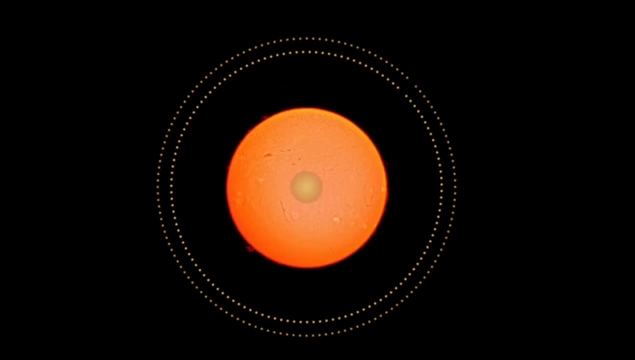 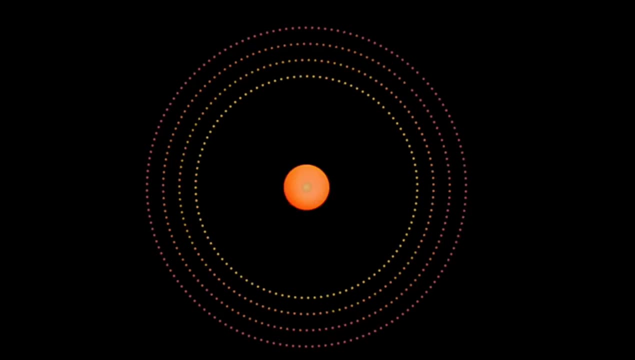 whilst it swells up on the outside. As the outer layers of the star grow larger, they cool off and become reddish in colour. A red star is cooler at its surface than a white star. Astronomers call these type of stars red giants. 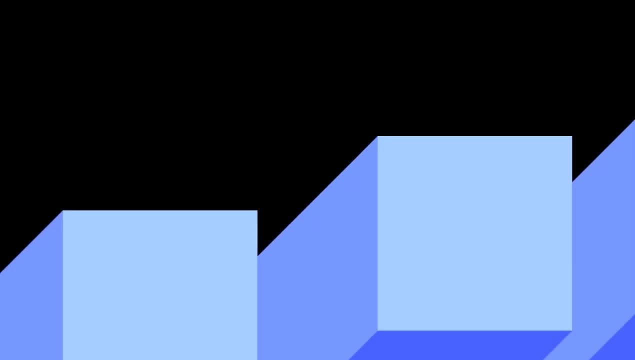 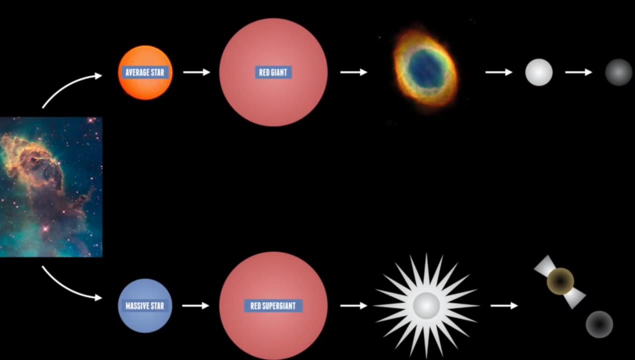 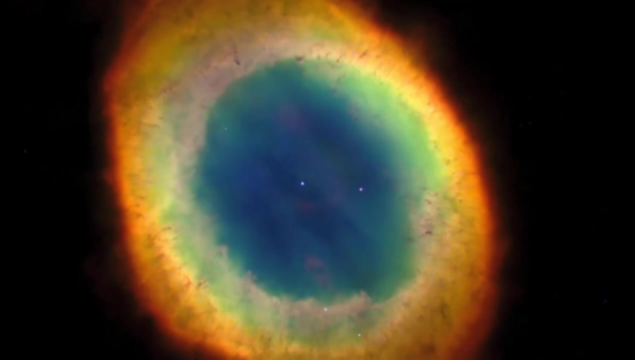 And they can become as large as the orbit of Mars or even Jupiter. The low mass stars, which is our sun, have only a limited ability to squeeze their cores to continue the fusion processes. They experience a period of instability where their outer layers lift off. 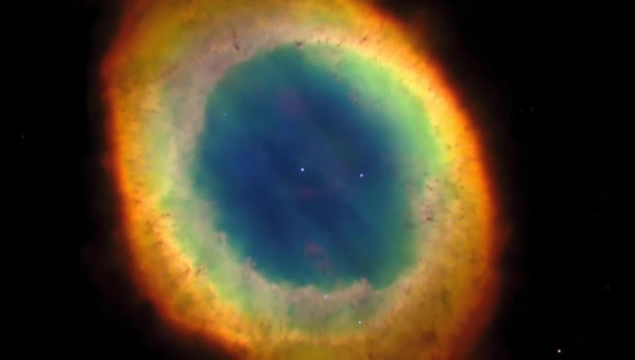 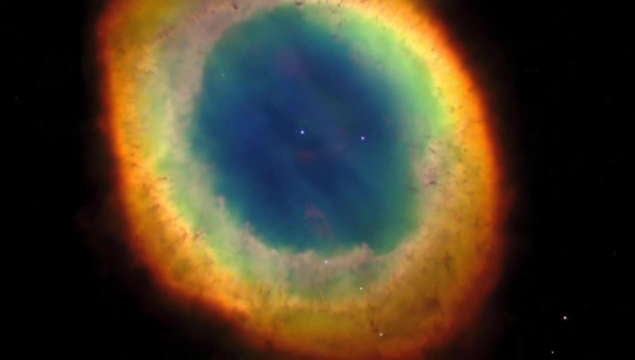 This period of instability for those stars produce some of the most beautiful objects in the night sky. As a star shreds its outer layers, the gas inside of it is illuminated by the light. This is called the red star. The red star is illuminated by the light of the collapsing star and glows in an array. 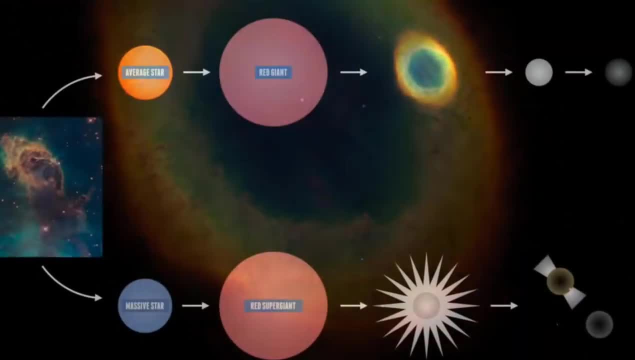 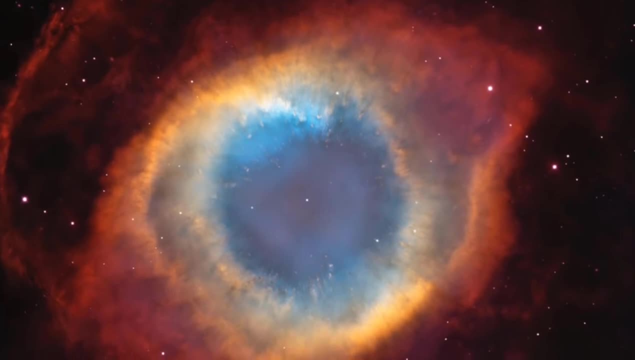 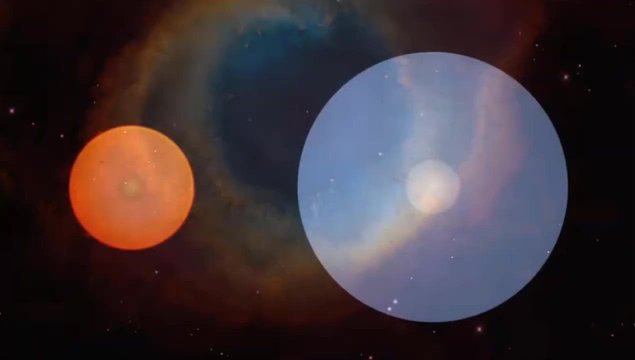 of colours. These are the last gasps of a dying star. These objects were named planetary nebulae because they resemble disks of planets, Although we now understand that they have no connection at all to planets, but the name, of course, has stuck. 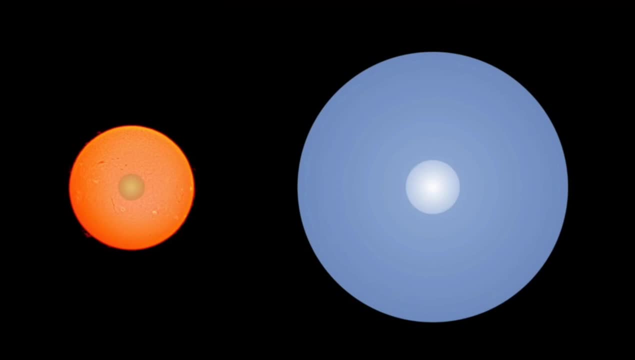 So, on the other hand, high mass stars have significant pressure and temperature at their cores. This means that they can continue the fusing process By using these newer, heavier atoms that they formed earlier. helium, carbon and oxygen are each in turn becoming fuel to make more energy for the star, and this is fighting. 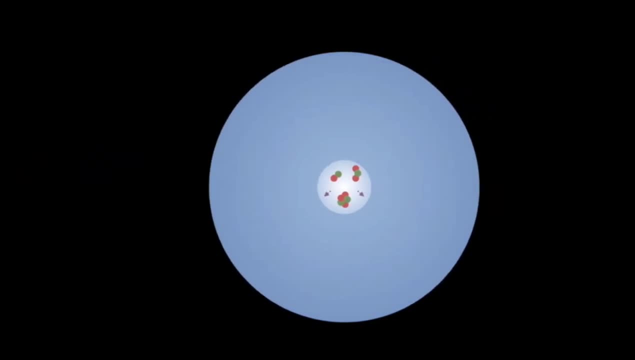 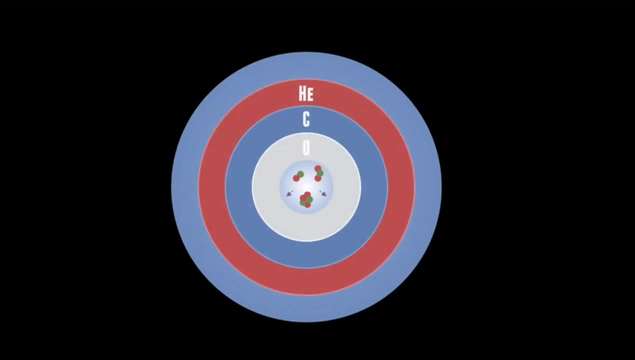 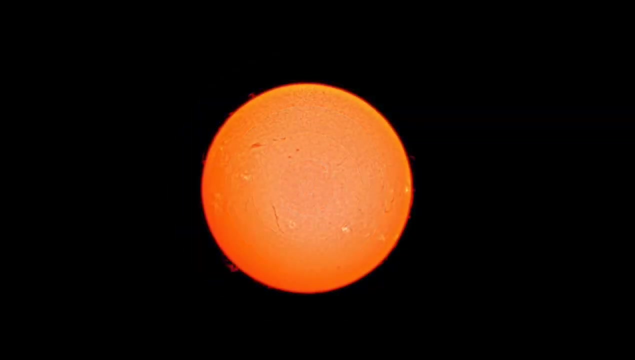 against the gravity, And this keeps the star stable, at least for a brief time. Eventually, however, the massive stars core becomes composed of simply iron, which sets off the final collapse. When low mass stars die, they collapse under their own weight until their centres act. 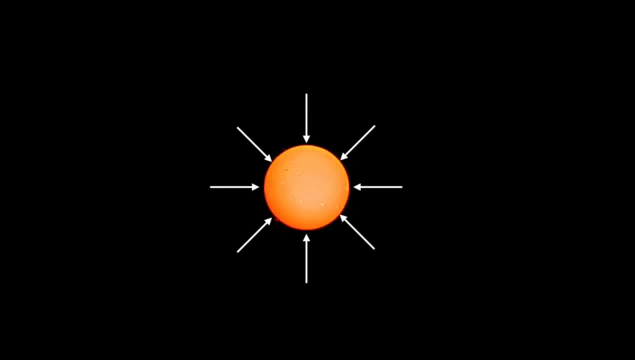 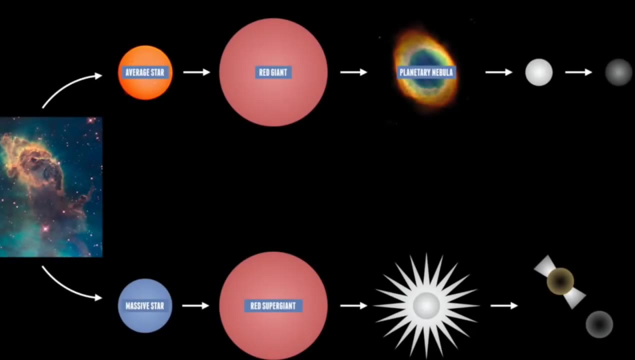 in the same ways, like a solid A star, like our sun, will collapse at the end of about twice the size of earth. These white, hot dying stars are called white dwarfs by astronomers. Perhaps the best known white dwarf orbits the brightest star in the sky, Sirius. 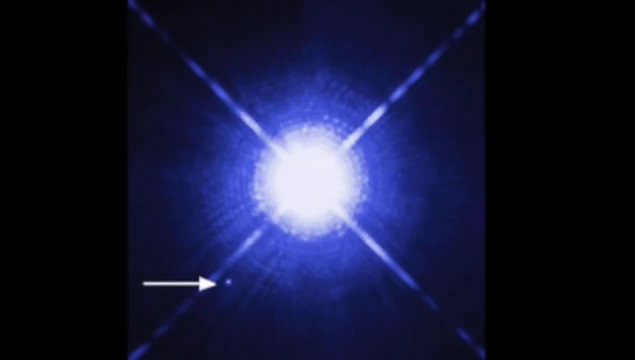 The star is called the white dwarf. Sirius is the brightest star in the sky. Sirius is the brightest star in the sky. Sirius is the brightest star in the air, But Sirius doesn't look as bright in this case. Sirius is the brightest star in the sky. 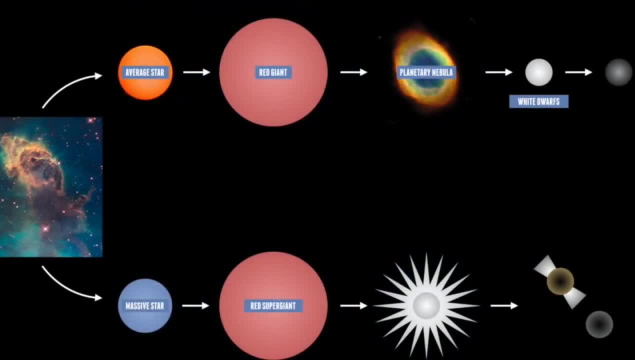 He does not look as bright in space as Sirius. It doesn't look as bright in space as Sirius did in핫use because when those big stars die, they don't are worth causing any trouble for the star to continue. Massive stars are very different in their ending. 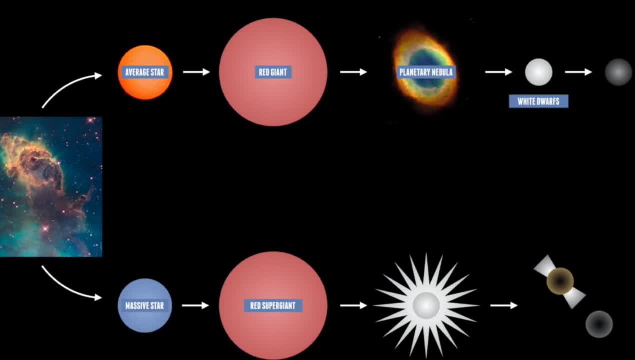 When the core of a massive star collapses, its powerful gravity takes it right through the white dwarf stage to produce one of two extremely bizarre objects, Either a neutron star or a black hole. In most cases, the rest of the star's jealous plane explodes. 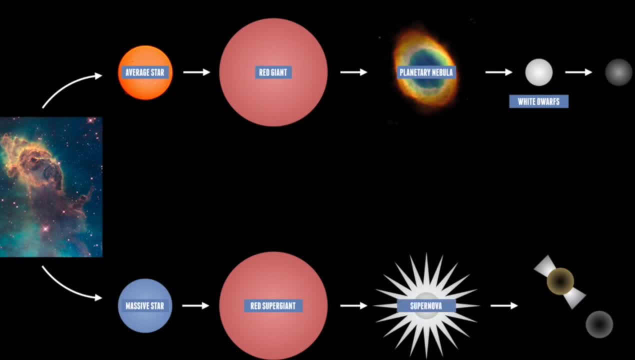 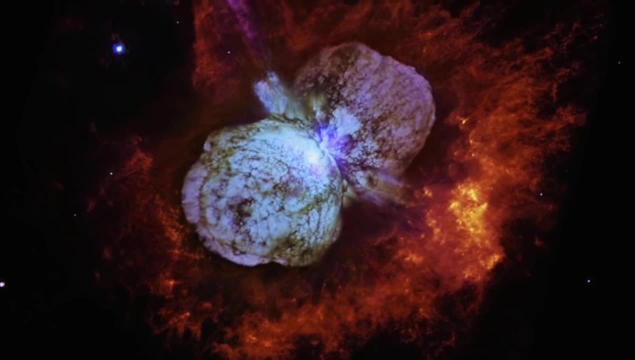 That star isâu seep or sides-by brings out an internal two-novalebrity and wind and BYD explosion called a supernova. Extreme versions of supernova explosions are sometimes referred to as hypernovae, and these produce gamma ray bursts, The most famous supernova in history. 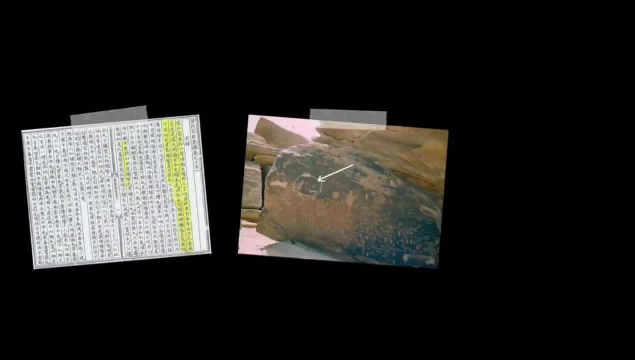 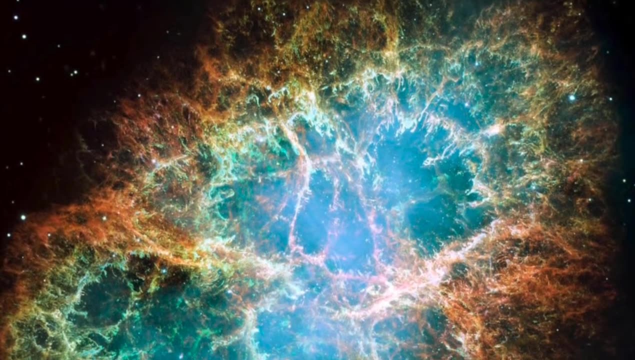 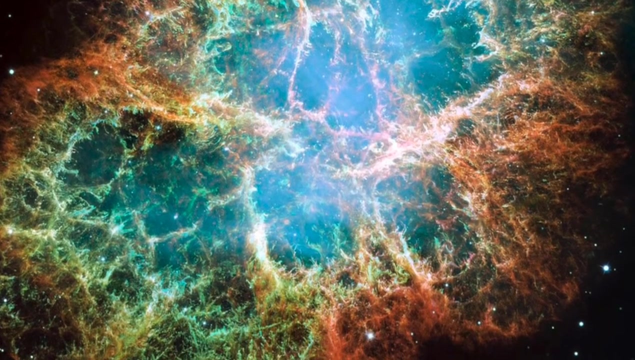 was in July 1054.. Records of this still survive from China all the way to North America. Seen today, roughly a thousand years later, its remnant is called the Crab Nebula and it is one of the interesting objects in the night sky. It can be found with a good pair of binoculars or a small 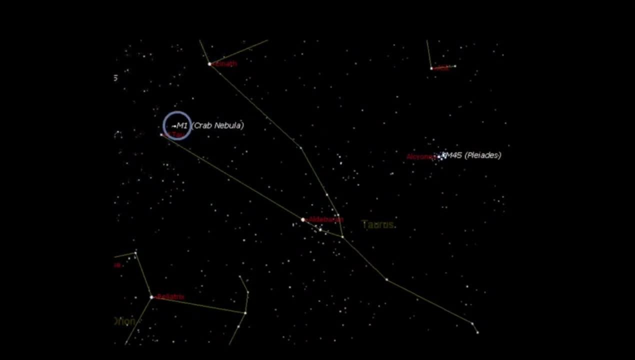 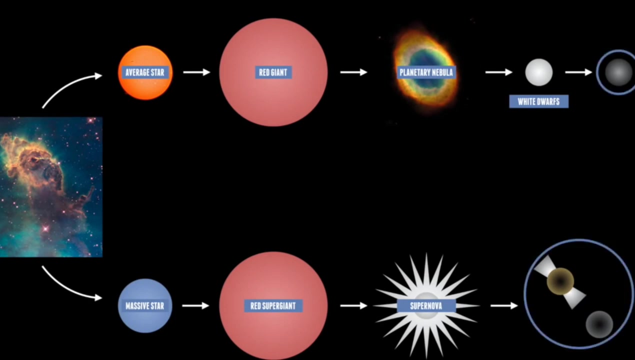 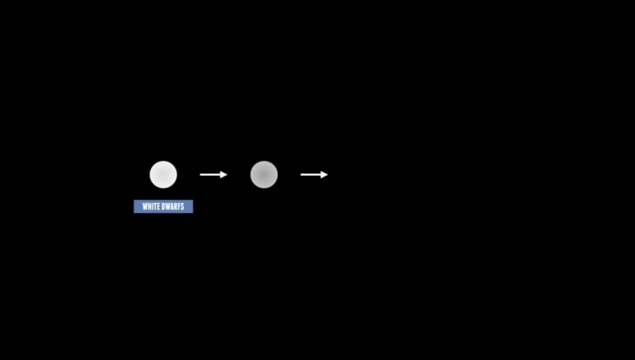 telescope in the constellation of Taurus. Near enough every star leaves a corpse. star corpses come in three bizarre varieties. A white dwarf fades away as billions of years pass. Since no energy is being produced inside of it and light is escaping off into space, the star's corpse slowly. 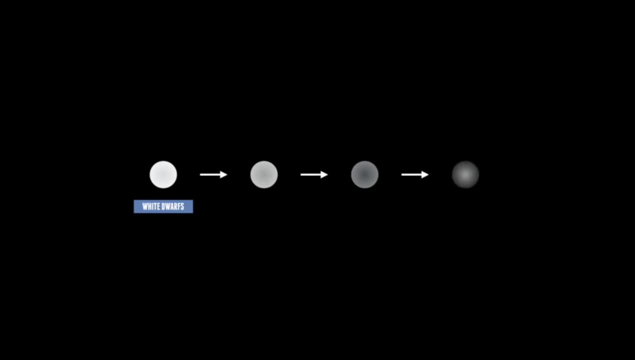 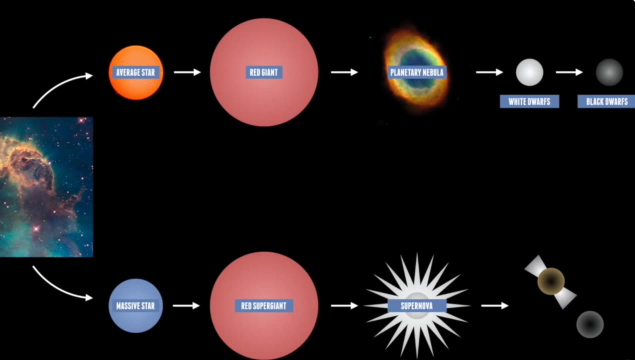 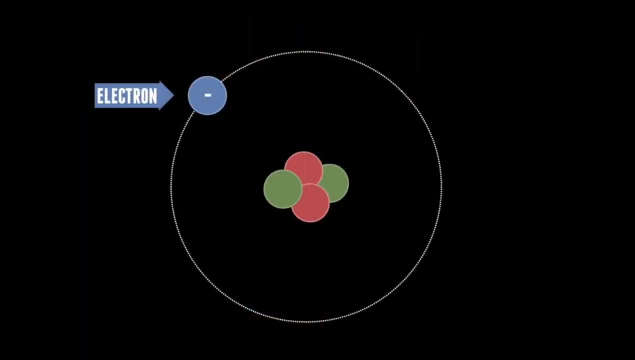 cools down. Astronomers call these corpses black dwarfs. A supernova explosion leaves behind a far more compressed corpse. The violent end to a massive star produces so much pressure that the star's core experiences a remarkable subatomic change: Electrons that are negatively charged particles.